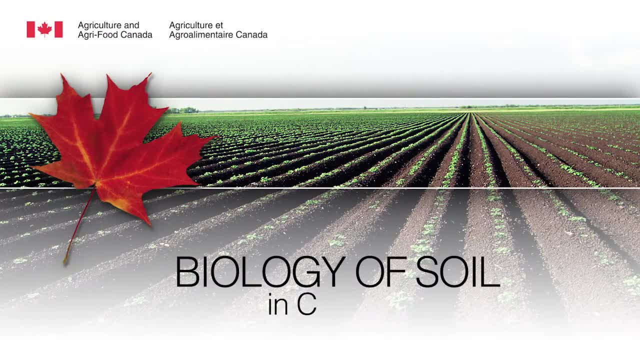 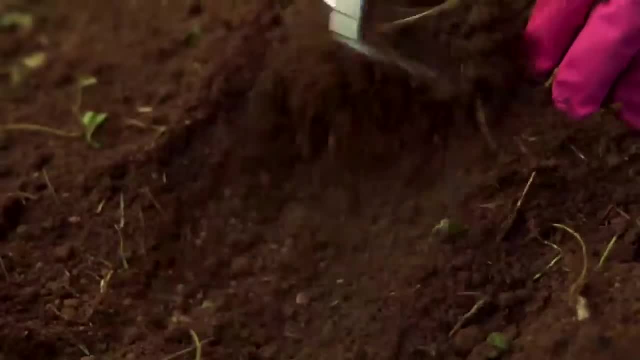 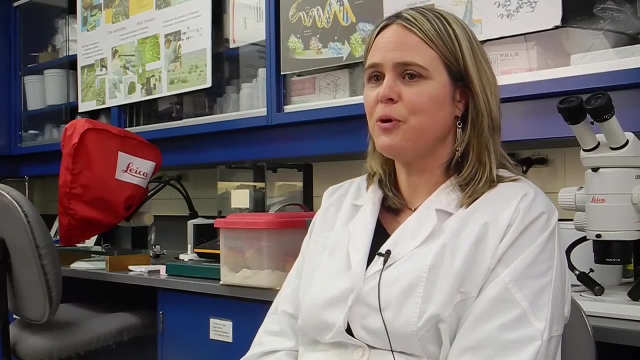 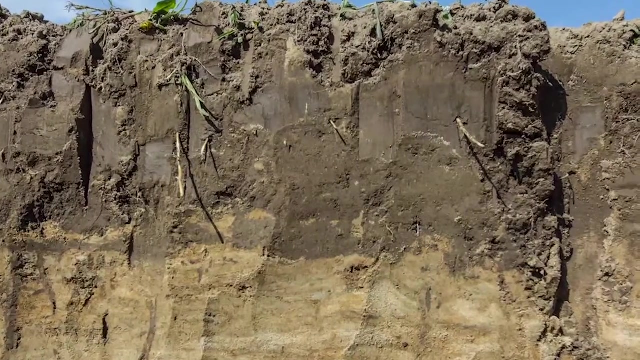 Soil is home of a large variety of organisms, going from a really large one- or larger, if you want, like insects and nematodes and earthworms, and to the very small, like bacteria, fungi. There are billions of organisms in every spoonful of soil. That means there are more organisms. 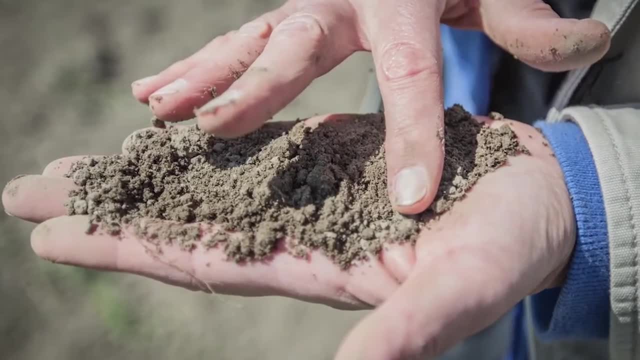 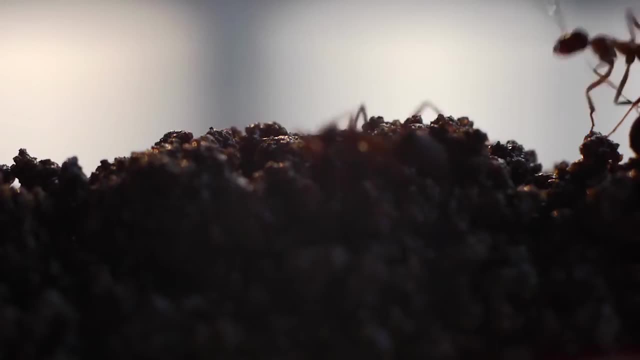 in a spoonful of soil than there are people on the planet. They are very small but they are very important to maintain the chemical environment of our world. Soils are actually quite alive. Organisms have a big role in soil. They basically affect. 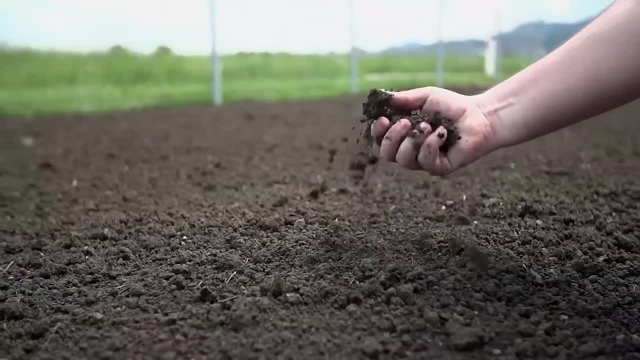 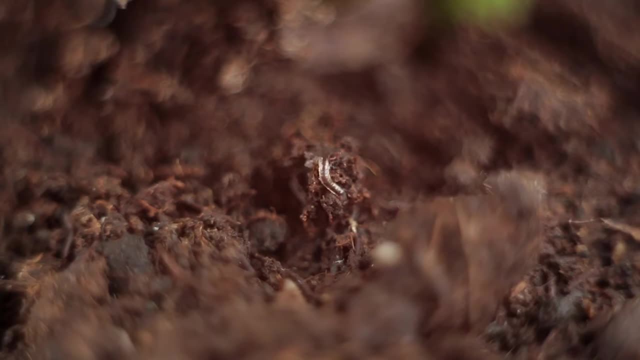 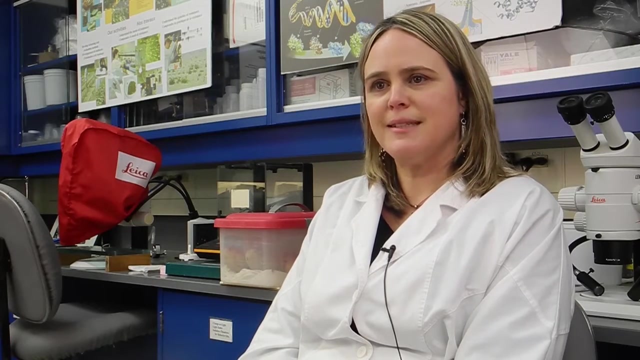 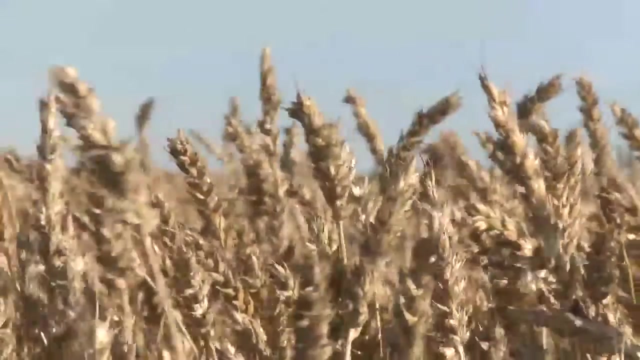 the chemical, the physical and the biochemical properties of soil. Basically, all organisms are involved in recycling. The process starts with larger organisms that will break down residue and animal waste in smaller fragments, and then the microorganism will further break down these bigger fragments in nutrients that can be taken up by plants. They play a vital 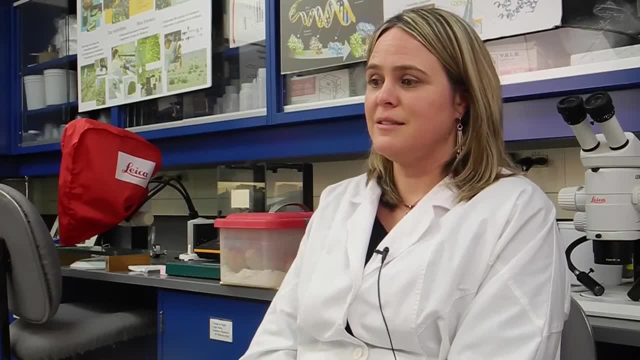 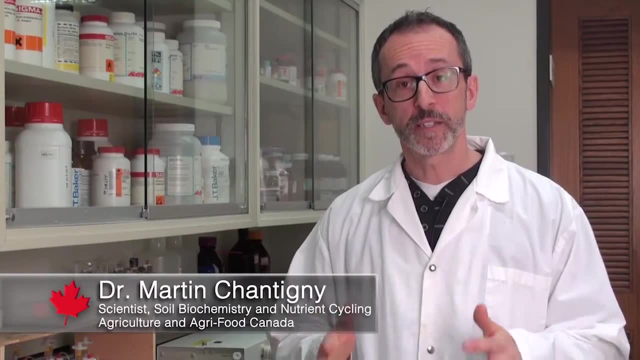 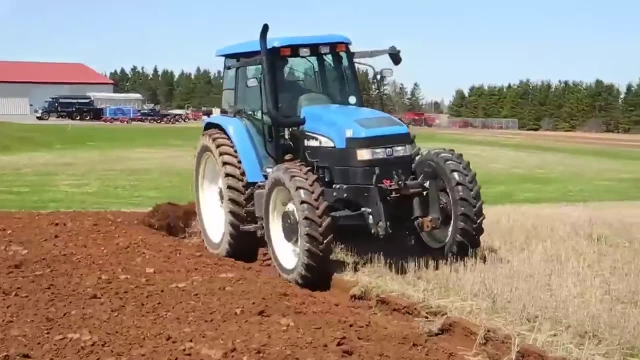 role in keeping our soil really healthy and ensuring that we're having a really good crop. Agricultural practices such as soil tillage, fertilization and crop rotation affect the abundance and functioning of soil organisms, And all of those organisms are very important for ecosystem functioning. 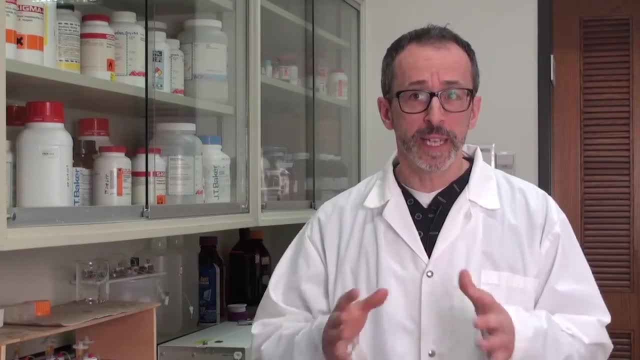 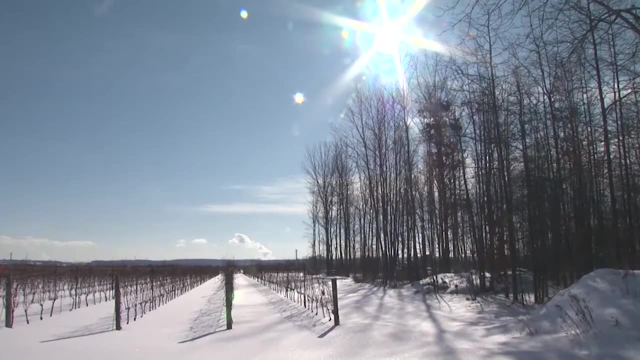 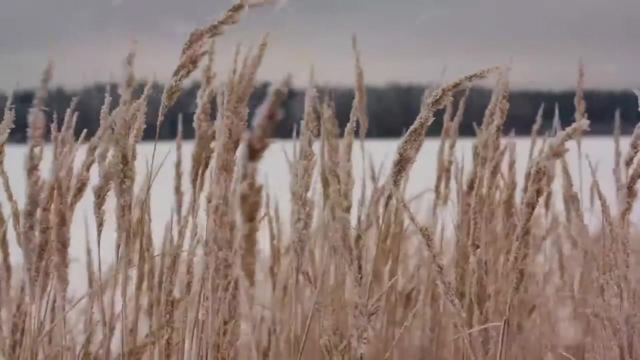 Soil biological activity is active at temperature well below freezing. Breakdown of plant materials- manure fertilizer- continues throughout winter, which affects nitrogen, phosphorus, carbon levels in soil and their fate in the ecosystem. Nutrient losses during winter may represent up to 90% of total annual losses, which is far from 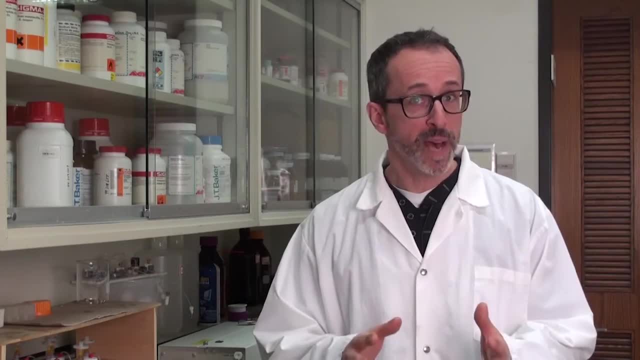 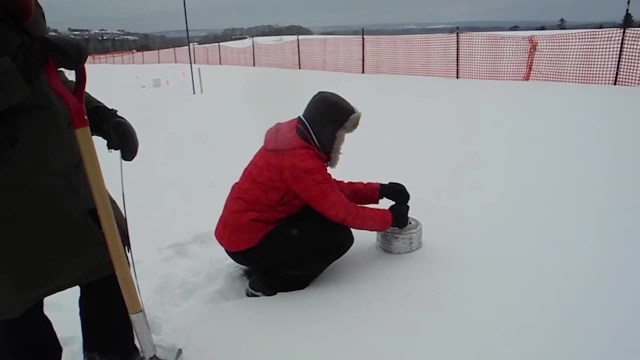 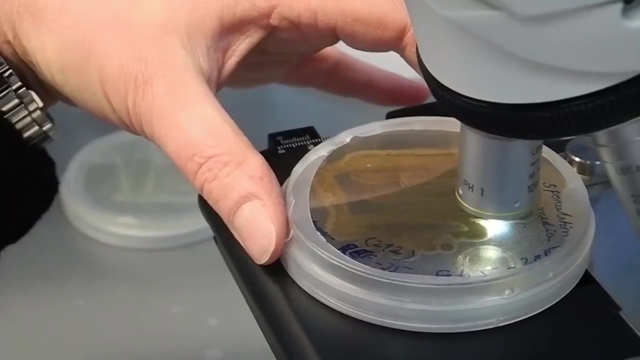 from being negligible. This has implication on the impact that fall application of manure and fertilizer may have on the environment. Our goal is to develop farm management practices that maximize retention of nutrients in the soil during winter, so we have a minimal impact on the environment.